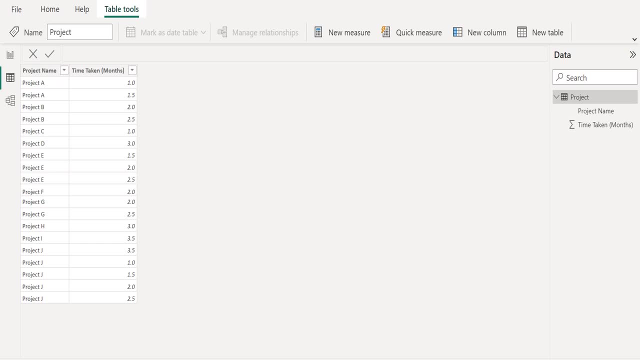 And in second column, time taken contains the duration of months to complete the respective project. Using this source data, we are going to calculate average per category with the help of DAX functions in Power BI. We will also explain you how we can achieve the average per category calculation using DAX functions in various methods with the help of Power BI. 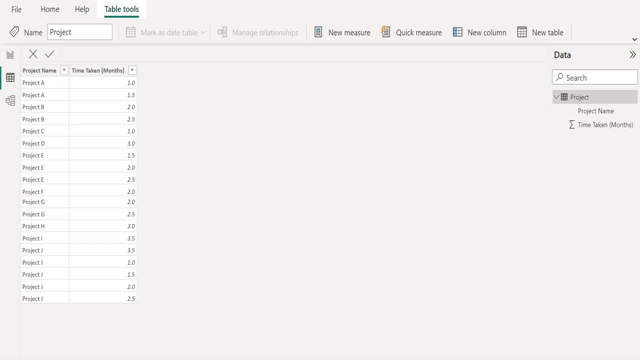 First step of calculated measure, calculated column and in quick measure. Then we will try to visualize this final output in table visual. Let's start with first method. We will use DAX functions in calculated measure to calculate average per category in Power BI. 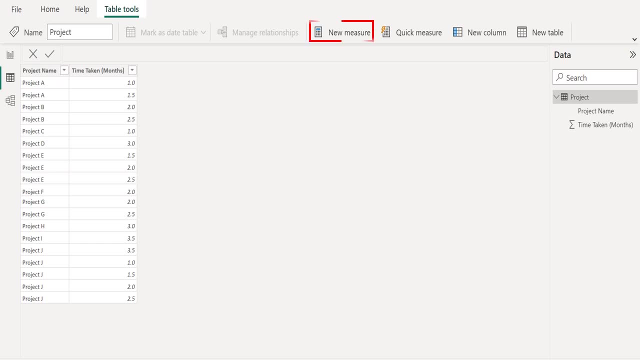 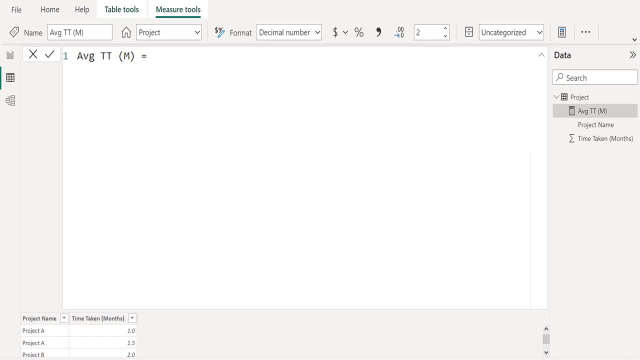 To create new measure. select new measure from Table Tools tab. The calculated results of measures of table will be shown in. the table are always changing in response to your interaction with your reports. Once you click on new measure, we can see the formula bar where we can write the DAX. 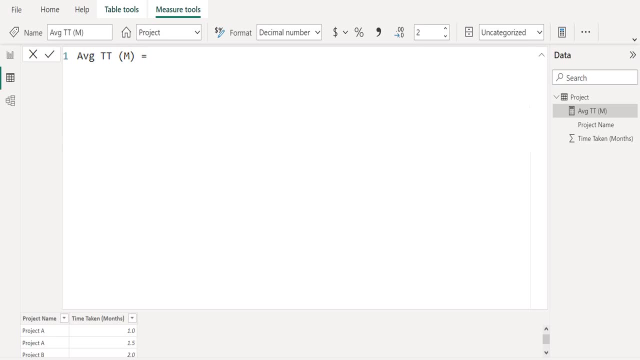 to calculate average per category in Power BI. We have renamed the new measure as Average of Time Taken is the short form of Average of Time Taken in Months. We will start writing the DAX function with calculate function. Calculate function is the often used DAX function in Power BI. 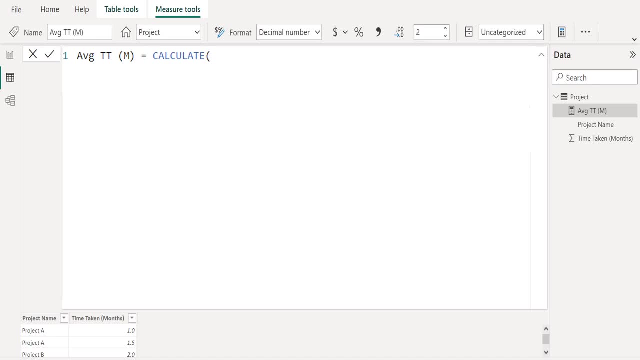 Even though calculate function cannot do anything, it works as a base function to apply other DAX functions in different scenarios. In this example, we want to apply a filter And find the average time taken for each project. In this case, we can use the calculate function to apply the filter and arrive at calculations. 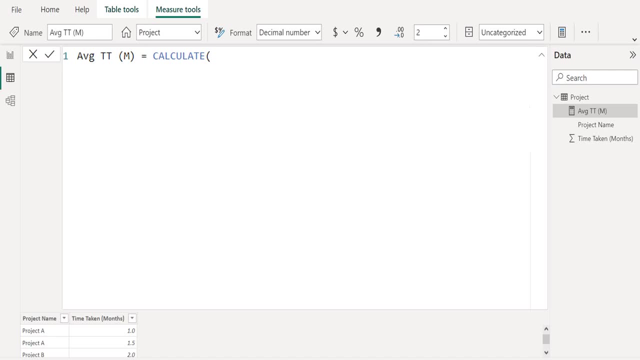 So the calculate function evaluates the expression given by the user, with all the applied filters. The syntax of the calculate function is calculate and expression parameter is nothing. but what is the expression we need to perform? Filter 1 parameter is based on the expression given. 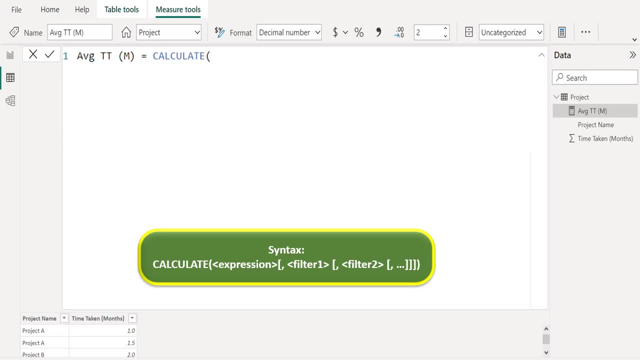 What is the filter we need to apply? Filter 2 parameter is based on the expression given. What is the second set of filters we need to apply? And close the parenthesis And expression is the first option. We need to add the time taken months. 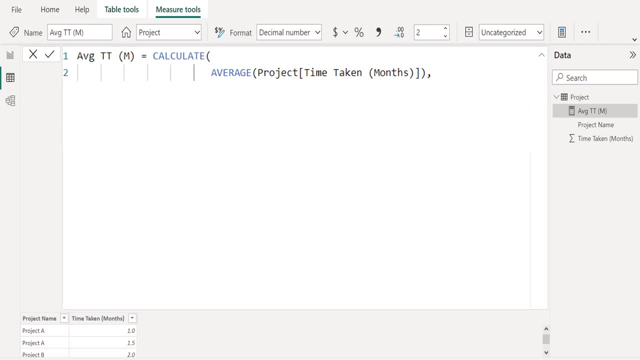 We need to add the time taken months. But what is the second option? in order to add the time taken months, we need to add a gallon of liquid isolated Soadd. a gallon of liquid, 4 grams of liquid, And outside that add a caffe plum. 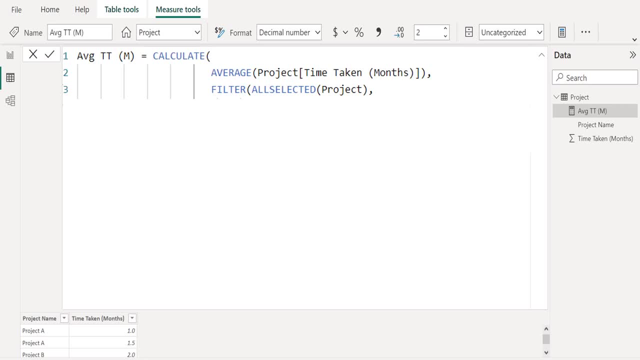 And the order of the filter set here is 1.. So adding a gallon will give us 1. another table or expression. the syntax of filter dax function is filter open parenthesis. in first parameter table input can be a table or it can also be an expression that results in a table. 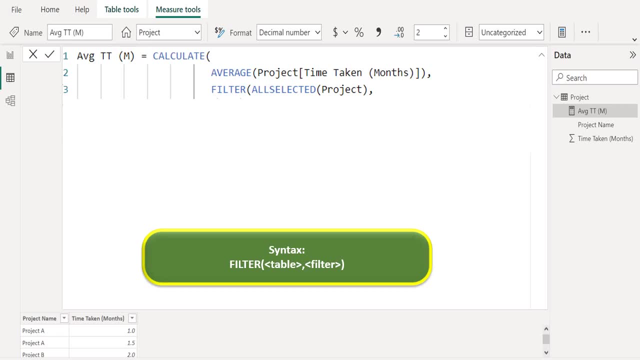 second parameter, filter, is a boolean expression that is to be evaluated for each row of the table. in table parameter of filter, dax function, we use all selected dax function. then select the project table. we need to select the project name column for filter expression and give the criteria as. 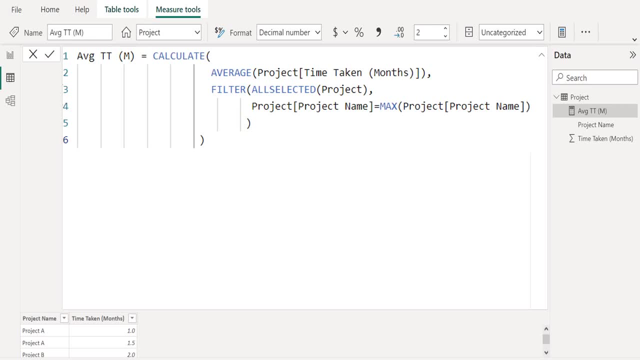 maximum of project name. we are done. close the parenthesis of filter dax function and calculate the filter dax function function and press the enter key to get the new measure. after you have created a new measure, it will appear in one of the tables on the field span which is found. 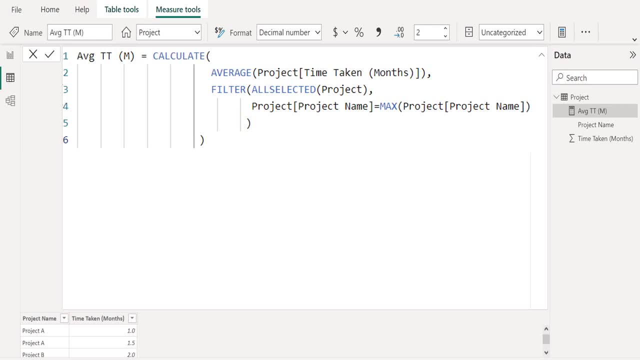 on the right side of the screen. power bi inserts the new measure into whichever table you have currently selected. while it doesn't matter exactly where the measure is in your data, you can easily move it by selecting the measure. you can use a measure like any other table column: just drag and drop it onto the 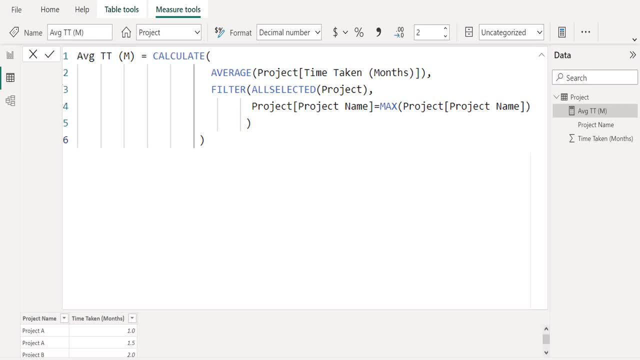 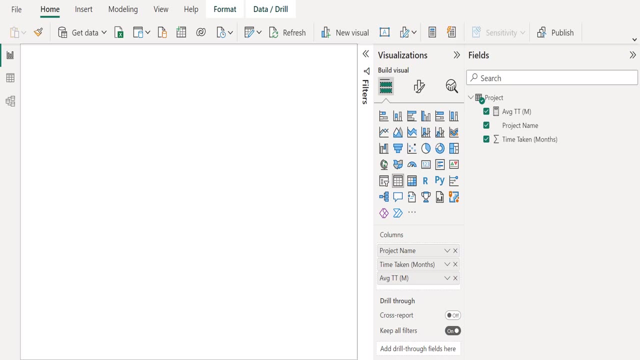 report, canvas or visualization fields. let's visualize the output in table visual. to create table, select table visual from visualization section and drag project name, name, time taken and newly created measure average time taken to columns of the table visual. Now table visual looks like this: 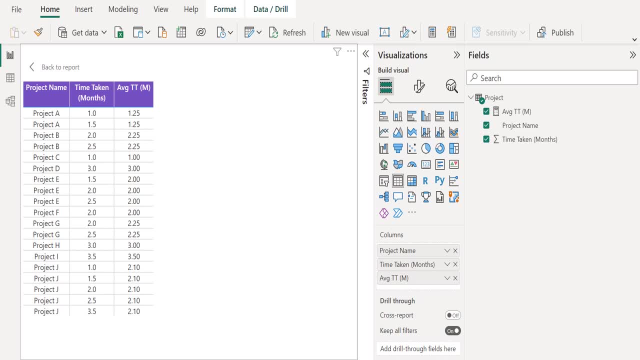 We can see the average per category in 3rd column. Project A, total time taken is 2.5 and it is divided by 2 because it contains 2 entries, and the average time taken of project A is 1.25.. For project J, total time taken is 10.5 and it is divided by 5 because it contains 5 entries. 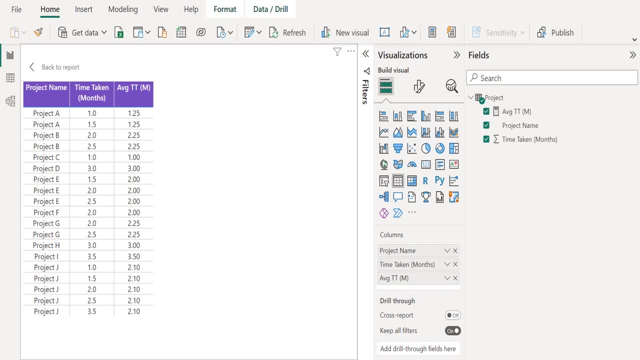 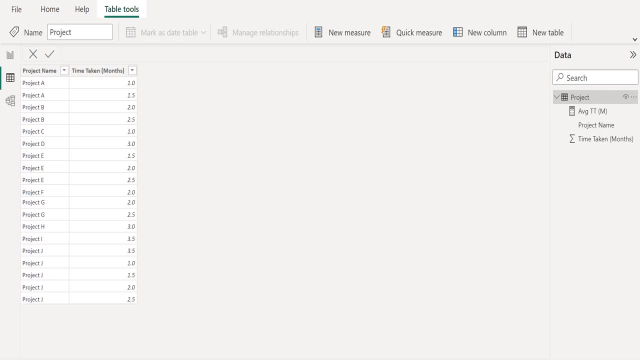 and the average time taken of project J is 2.1.. Second method: we will use DAX functions in calculated column to calculate average per category. To create new column, select new column from table tool tab. With calculated columns you can add new data to a table already in your model. 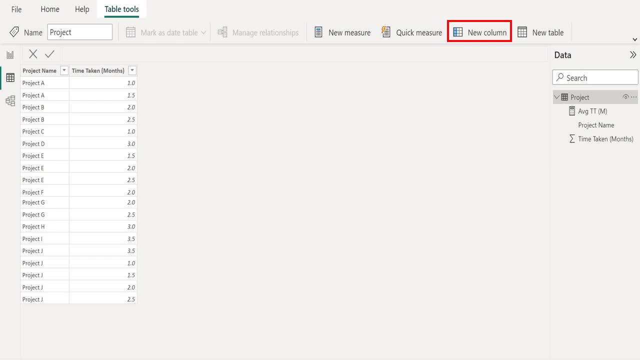 But instead of querying and loading values into your new column from a data source, you create a data analysis expressions formula that defines the column's value. Calculated columns you create appear in the fields list just like any other field, But they will have a special icon showing its value or the result of a formula. 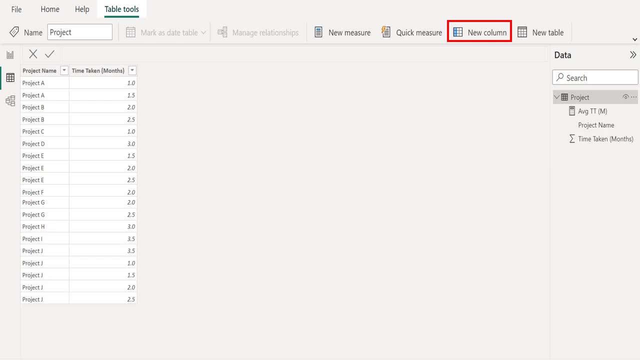 You can name your columns whatever you want and add them to a report visualization, just like other fields. Calculated columns calculate results by using DAX, a formula language to work with relational data, like in Power BI desktop. In Power BI, when you create a DAX formula for a new column, it will calculate a result. 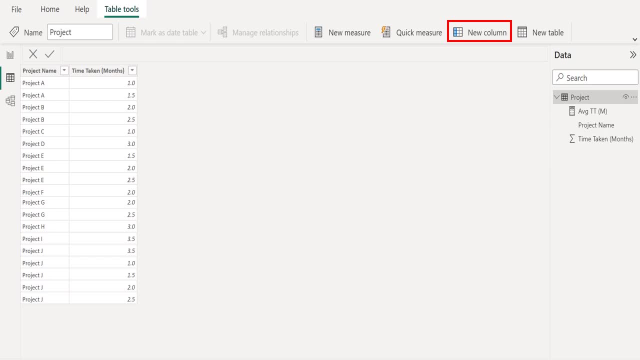 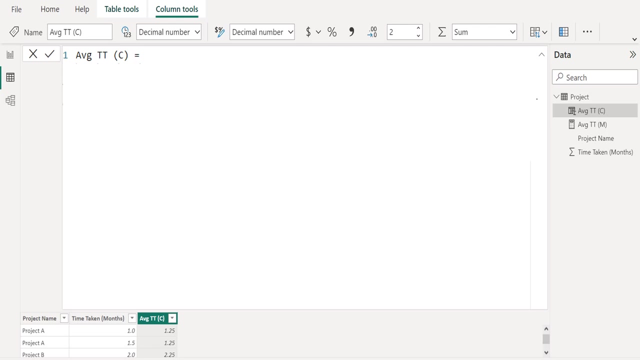 for every row in the table. Column values are recalculated as necessary, like when the underlying data is refreshed and values have changed. We have renamed the calculated column as Average of time taken. open parenthesis C indicate that it is the calculated column and is the short form of Average time taken. 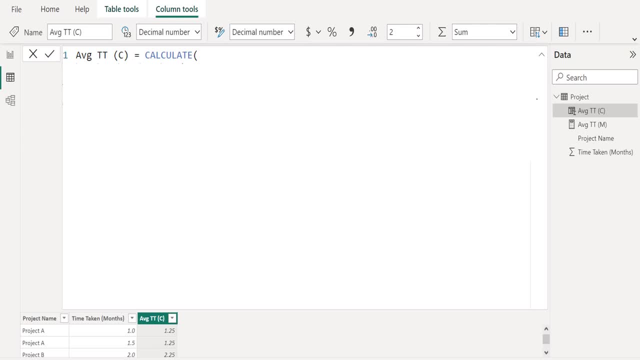 We will start writing the DAX function with calculate function and expression is the first option. We need to add the time taken, months average in this example, So open the average function. The column name We need to average is the time taken. column from project table. 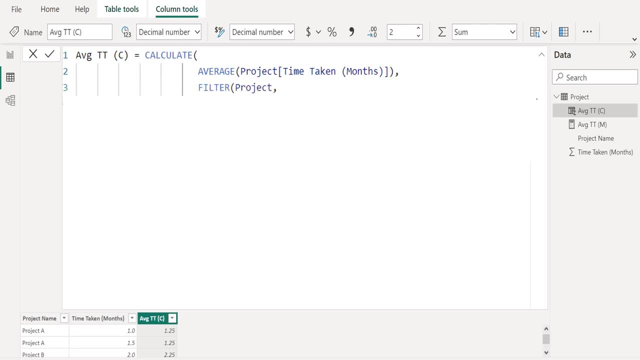 So choose the respective column, Use filter function which returns to table that represents a subset of another table or expression. The table we refer to is the project. So first choose the table name to filter. We need to select the project name column For filter expression and give the criteria, as earlier, of project name. 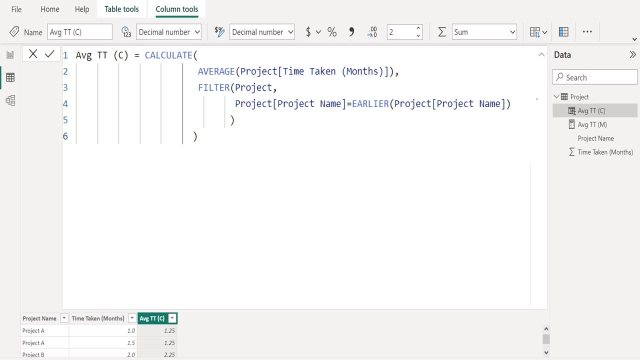 Earlier function returns the current value of the specified column in an outer evaluation pass of the mentioned column. Earlier is useful for nested calculations where we need to use a certain value as an input and produce calculations based on that input. Input an input In Microsoft Excel, we can do such calculations only within the context of the current row. However, in DAX we can store the value of the input and then make calculations using data from the entire table. 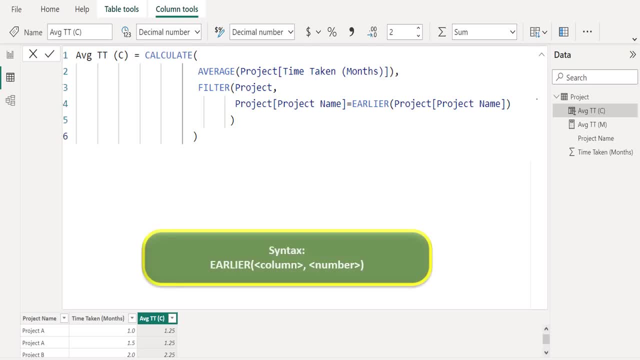 The syntax of earlier DAX function is: earlier open parenthesis. first parameter column is a column or expression that resolves to a column. second parameter number is a positive number to the outer evaluation pass and close the parenthesis. Earlier succeeds if there is a row context prior to the beginning of the table scan. 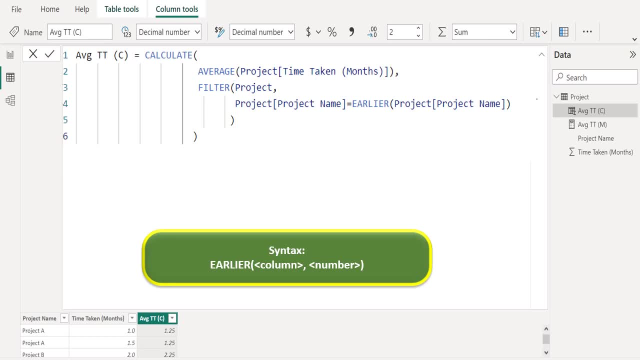 Otherwise it returns an error. The performance of earlier might be slow because theoretically it might have to perform several operations. that is close to the total number of rows in the column, Same number which will repeat for syntax of the expression. For example, if you have 10 rows in the column, approximately 100 operations could be required. 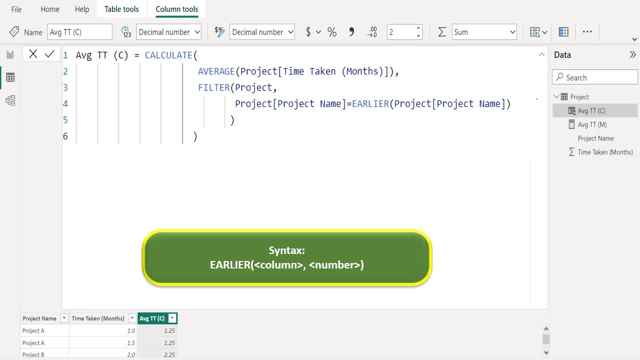 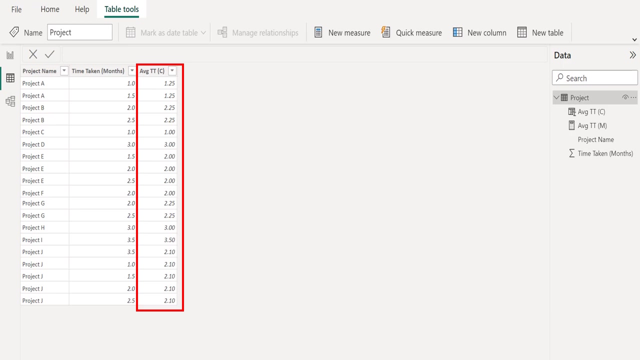 If you have 100 rows then close to 10,000 operations might be performed. We have done close the parenthesis of filter DAX function and calculate DAX function and press the Enter key to get the new calculated column. We can see the new calculated column with the values of average per category. 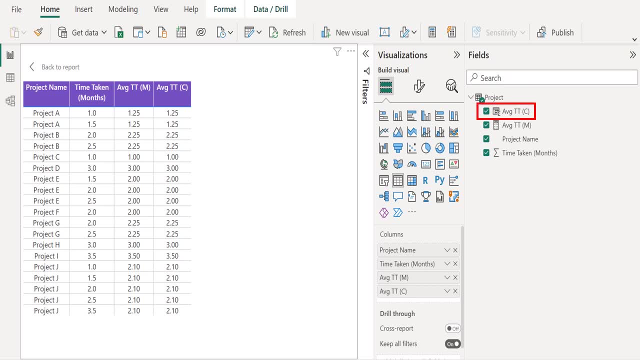 Drag calculated column from the column to the new calculated column. Drag calculated column from the column to the new calculated column from source and place it in columns. In table visual, fourth column shows the result of calculated columns and it is like the result of calculated measure in. 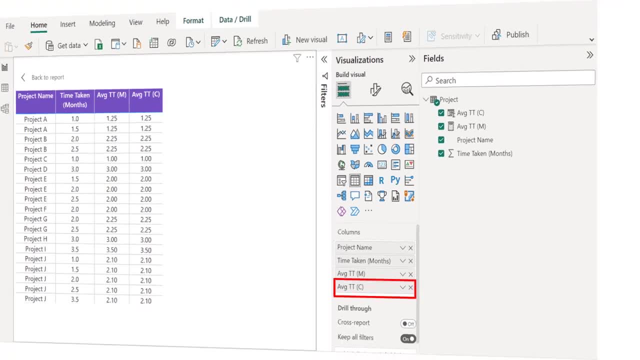 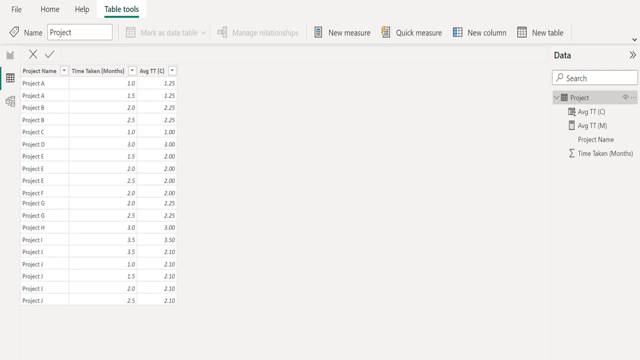 the third column So far we saw how to calculate average per category using DAX function in measure and calculated column. Next we will see the disadvantage of quick measure in calculating average per category. To create quick measure, select quick measure from table tools tab. We can use quick measures to quickly and 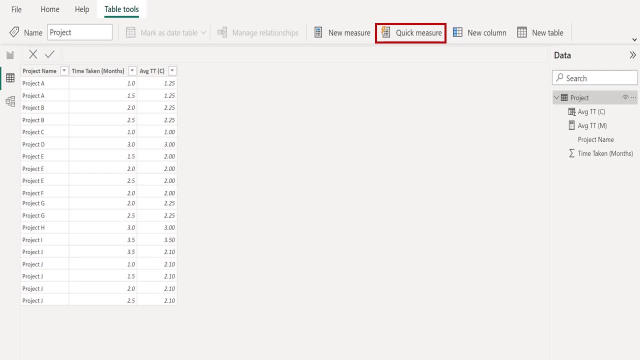 easily perform common, powerful calculations. A quick measure runs a set of data analysis expressions behind these scenes, then presents the results for you to use in your report. You don't have to write the DAX by default. It's done for you based on input you provide in a dialog box There. 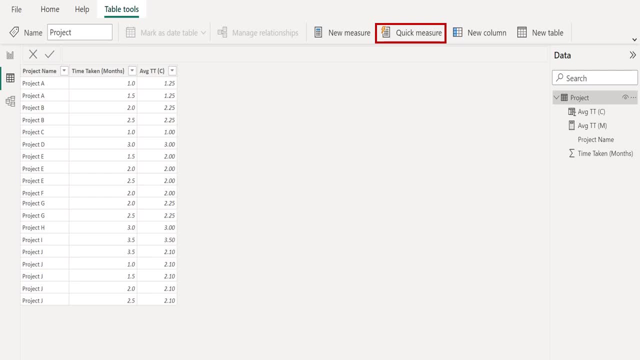 are many available categories of calculations and ways to modify each calculation to fit your needs. When we select new measure, the quick measures window appears. It allows us to choose the calculation we want and the fields to run the calculation against. Choose the select a calculation field to. 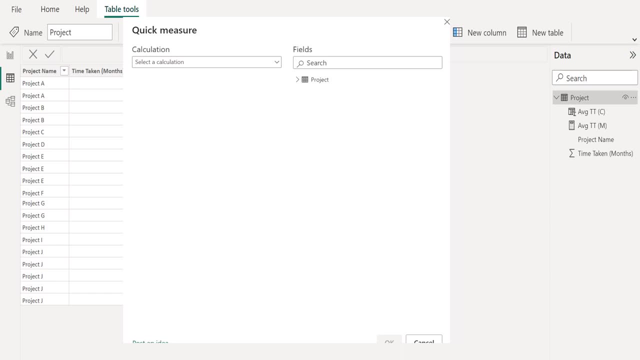 to see a long list of available quick measures. In calculation field, select the average per category. then select time taken column from source table and place it in base value and change the aggregation to average of time taken. Next select project name from source table and place it in category. click ok to confirm the changes we have done so far in. 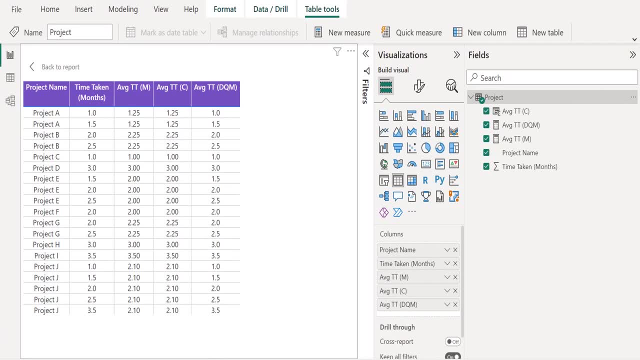 this window. We have renamed the quick measure as average- tt- open parenthesis, dqm- closing parenthesis and drag it to columns of the table. visual: Now we can see the quick measure results in 5th column. If you notice, the results of quick measure is don't meet our requirement. It only replicates. 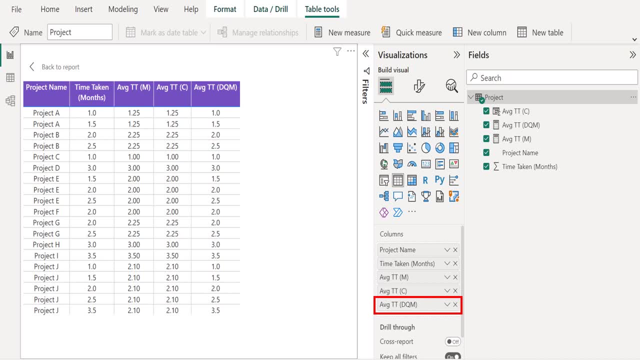 the same data of time taken column. This is the disadvantage of quick measure in calculating average per category in Power BI. These are the three different ways to calculate the average per category in Power BI. If this video helps you, please like and share this video. 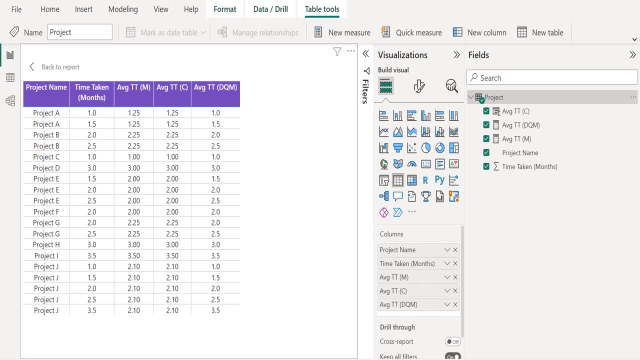 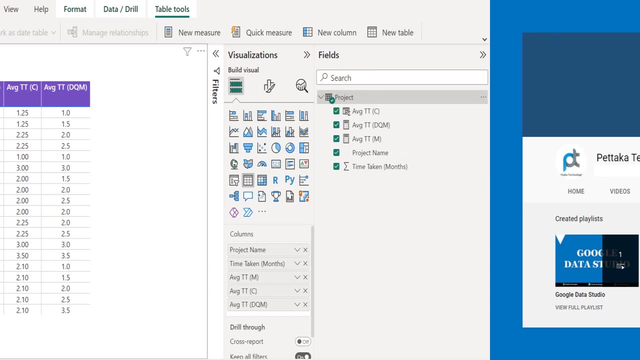 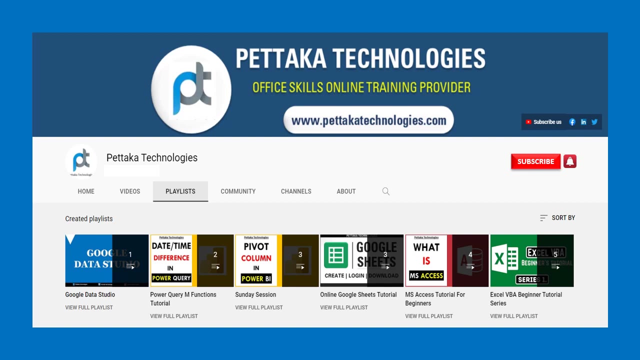 Ask your questions or share your feedback in below comments section. To watch more videos like this, visit our official youtube channel petaka technologies To book your slot for online training. visit our official website petakatechnologiescom To get notifications on upcoming videos. subscribe to this channel and activate bell icon. 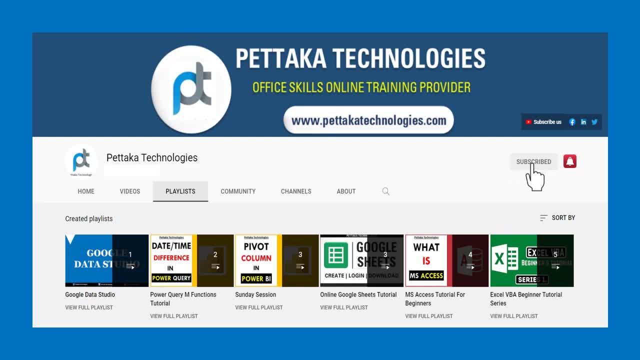 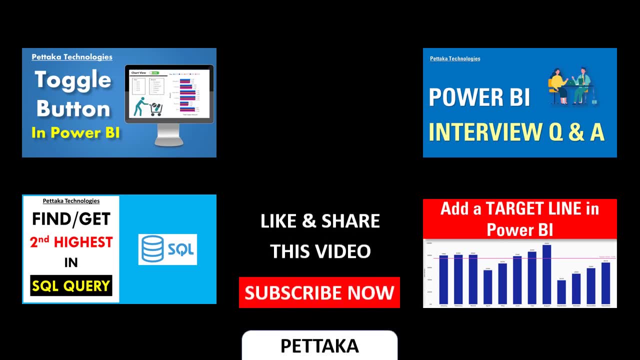 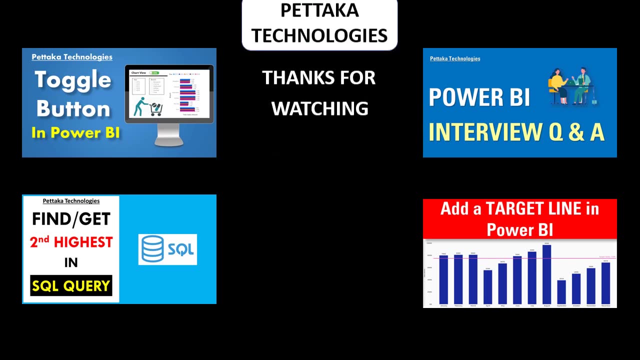 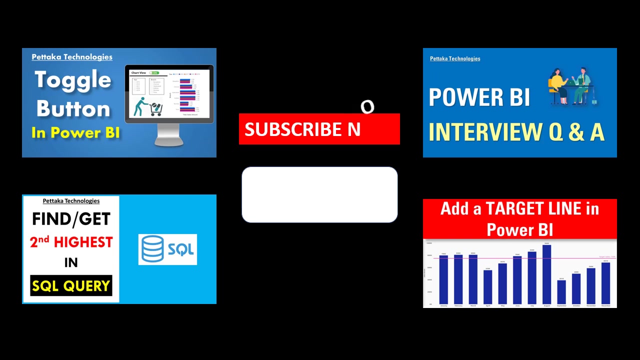 That's all for this video. Thanks for watching. Have a great day.